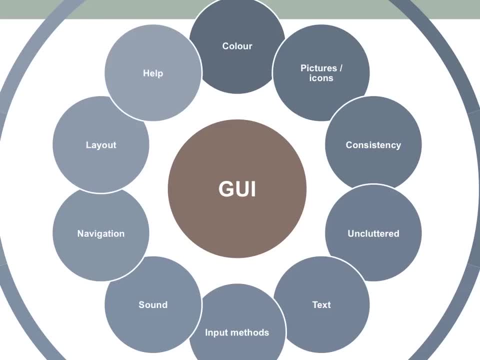 If you click a button in the other, you should click a button in the other. If you click a button in the other, you should click a button in the other, And the navigation structure shouldn't change from page to page. It's also important for the user interface to appear uncluttered. 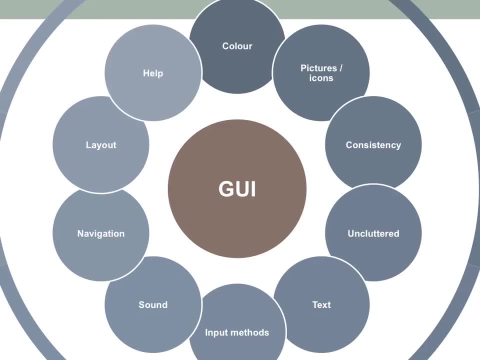